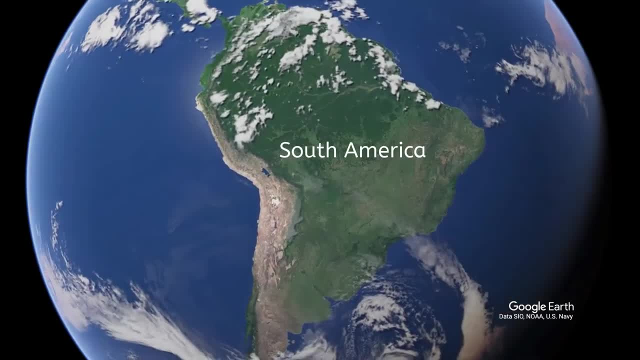 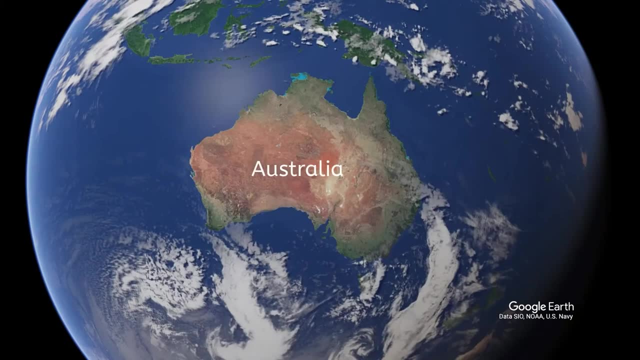 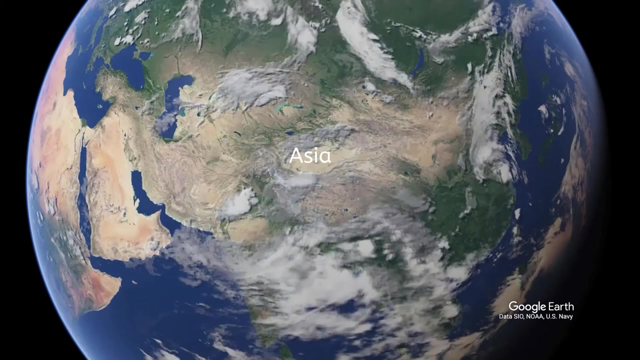 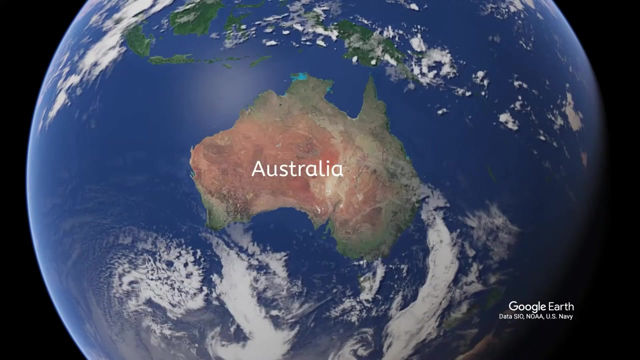 North America, South America, Europe, Africa, Asia, Australia and Antarctica. An eighth continent, Oceania, is sometimes added to that list. Asia is the largest continent, at 17.21 million square miles, and Australia is the smallest, at 2.97 million square miles. 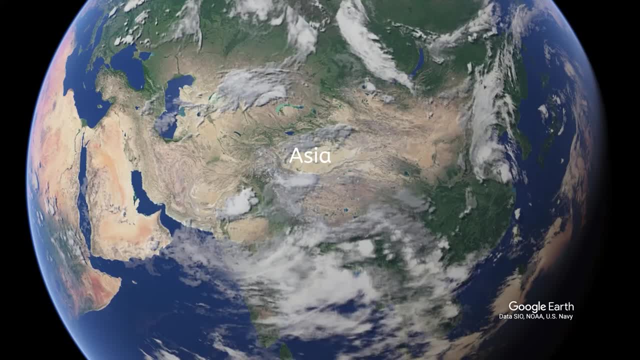 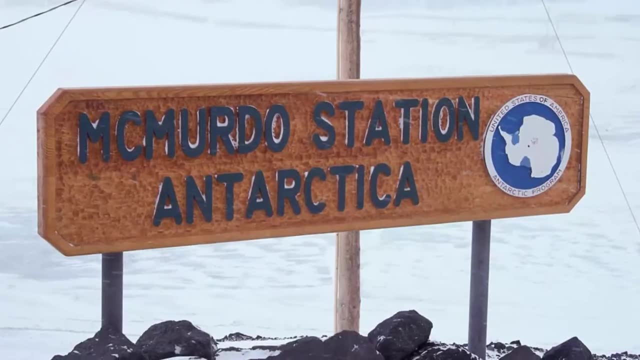 Asia is also the largest continent in terms of population, at over 4.4 billion people. The least populated is Antarctica, which has research stations but no permanent residence, and yet has somehow been the birthplace of at least 11 children since 1978. 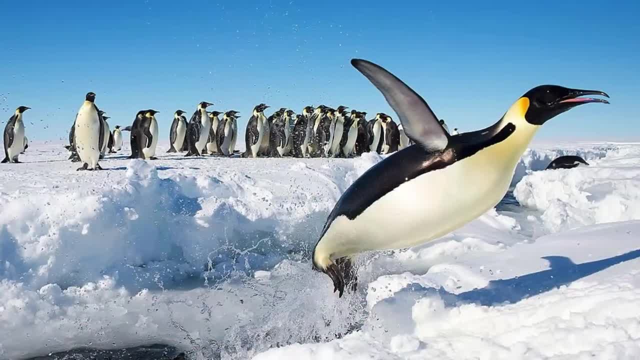 Also, Antarctica has no time zones, contains 90% of the world's population and is the largest continent in the world. Oceania holds 70% of the world's ice, holds 70% of the world's freshwater in the form of glaciers. 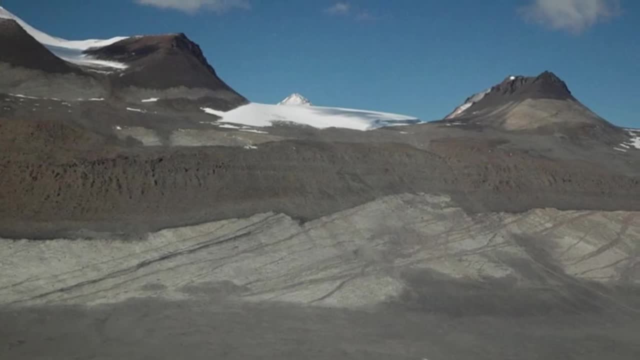 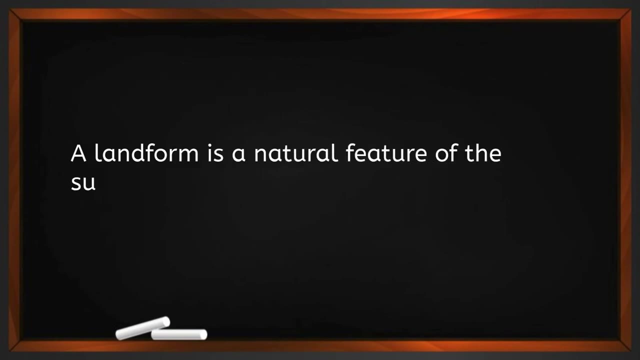 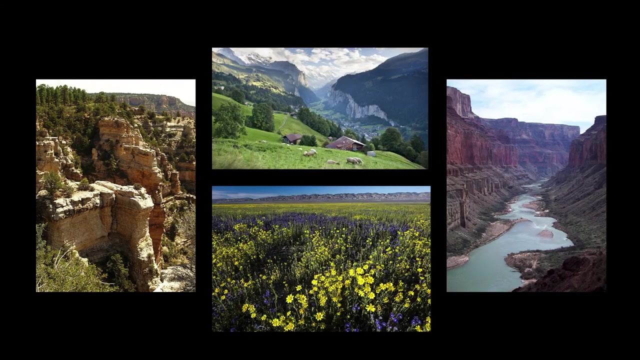 and has a number of ice-free valleys that haven't received rain in 2 million years. Continents are made up mostly of landforms. A landform is a natural feature of the surface of the earth. A few examples are mountains, hills, plateaus, canyons, valleys and plains. 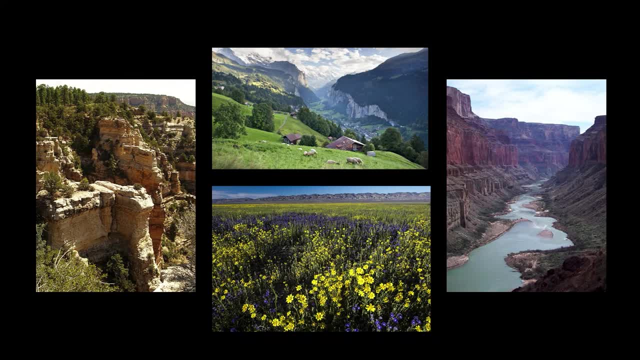 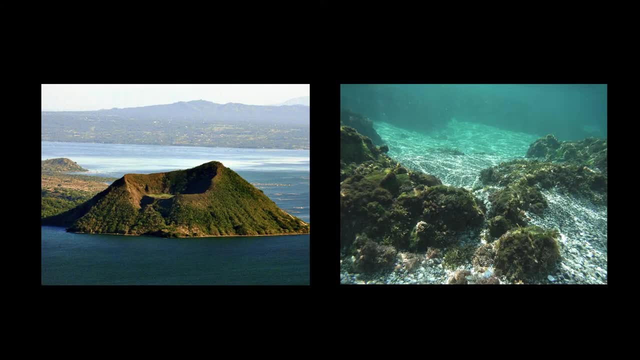 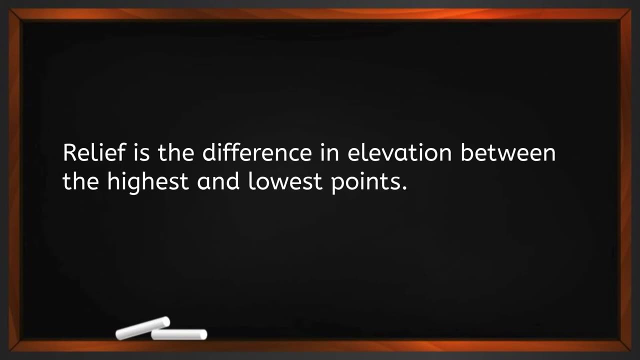 Landforms can also include shoreline features and submerged features such as bays, peninsulas, seas and mid-ocean ridges. Typically, landforms are classified according to differences in relief, which is the difference in elevation between the highest and lowest points. 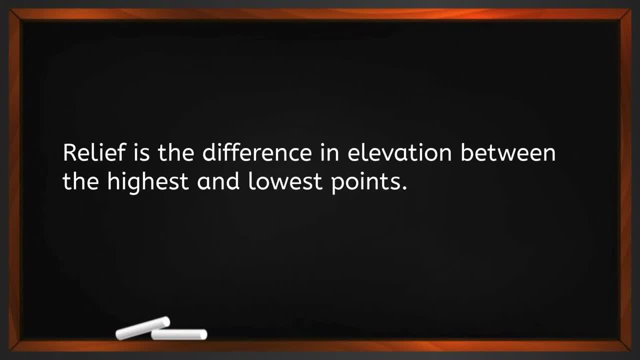 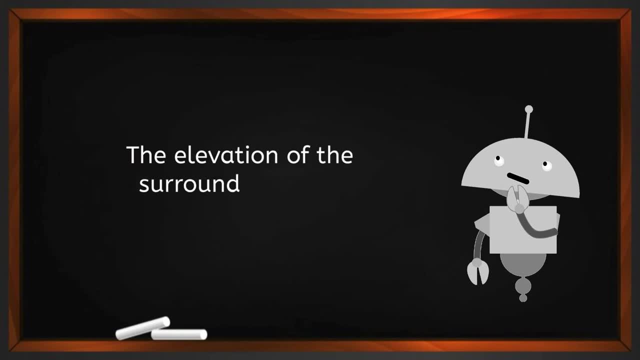 Mountains have high relief. Hills, which are typically lower and rounder, have lower relief. So wait, what's the actual difference between a mountain and a hill? The elevation of the surrounding land determines that. For example, a mountain in Ireland which 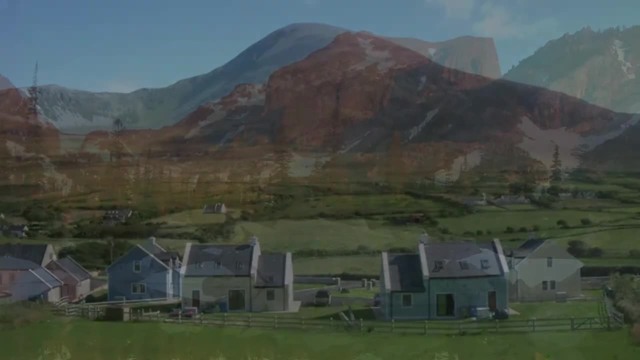 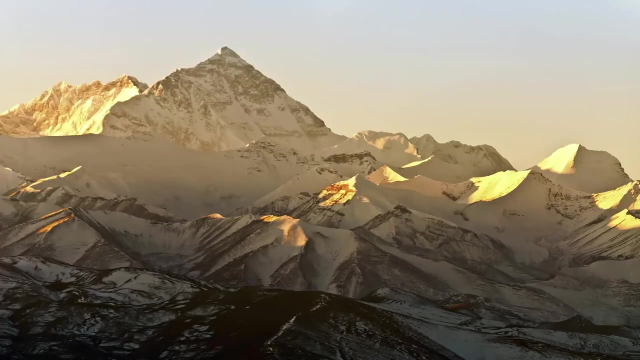 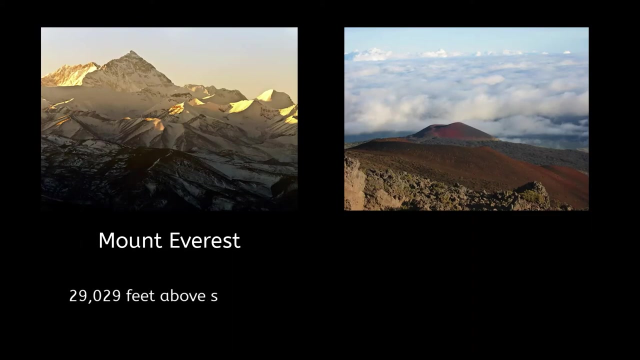 sits at a relatively low elevation might be considered a hill in the Rockies which sit at a relatively high elevation. So what's the highest mountain in the world? Everest, right? Well, no, It's Mauna Kea in Hawaii. Mount Everest stands at 29,029 feet above sea level. 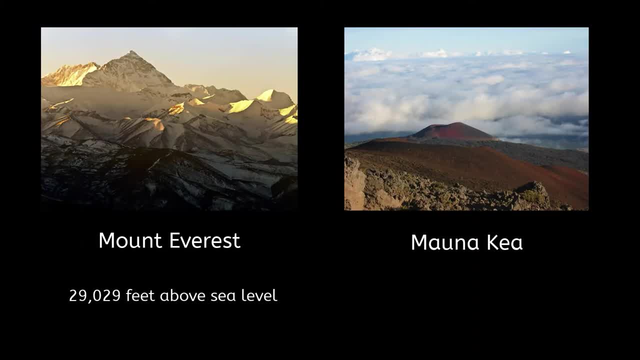 Very impressive. Mauna Kea, on the other hand, stands only 13,796 feet above sea level, And yet it's nearly a mile taller than Everest. How is this possible? Because Mauna Kea extends 19,700 feet below the ocean. 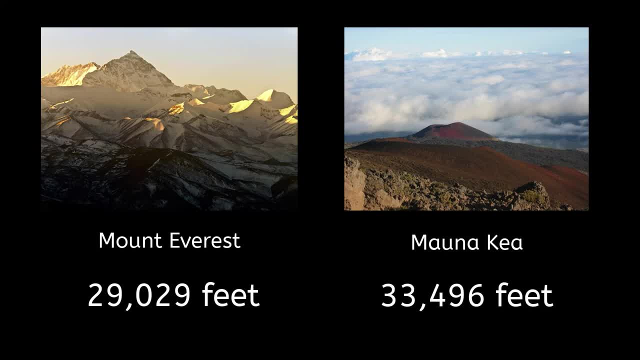 So where's the point? Well, the point is the highest point on the earth as measured from the center of the earth, Which puts Mauna Kea at a total height of 33,496 feet, And a part of the point is the highest point on the earth. 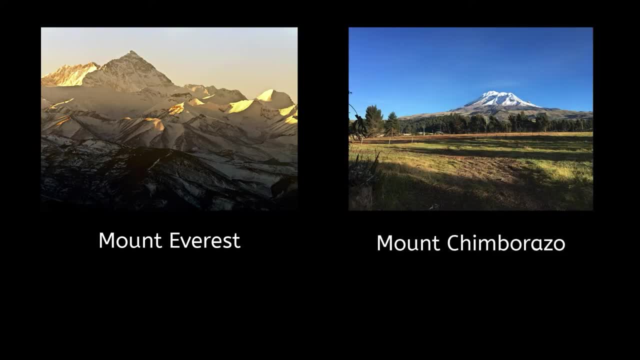 The highest point on the earth is Mount Chimborazo in Ecuador. Wait, what Everyone knows? Mount Everest is the highest point of the Earth, Right. Well, as we learned before, the belief that the earth is round rather than flat originated with the ancient Greeks and the notion that the earth is a perfect sphere. 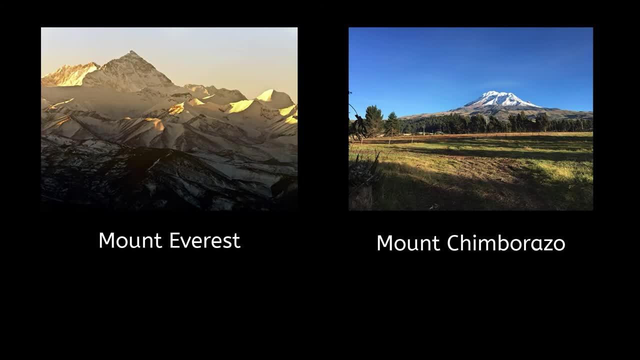 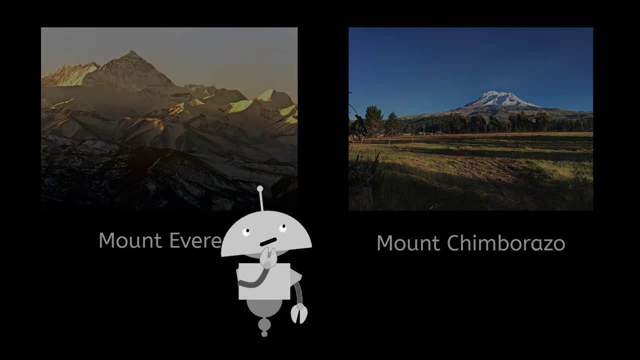 And the fact that it's actually round would be more accurate than a flat star. the Earth is a perfect sphere grew from that early hypothesis. But guess what? The Earth is not a perfect sphere. Wait what? The Earth isn't a perfect sphere. No, it's not, It's. 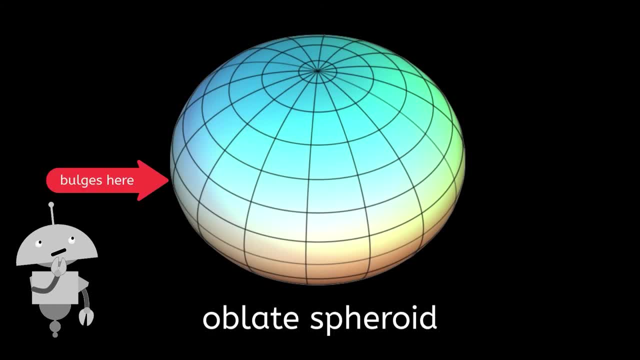 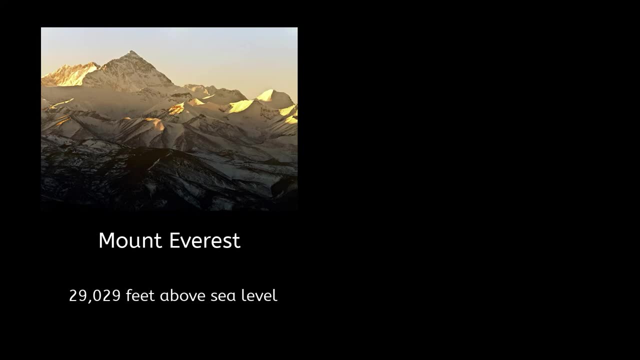 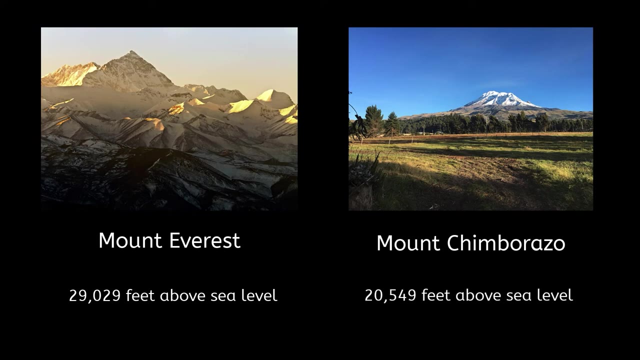 an oblate spheroid, which means it bulges at the equator and flattens at the poles as a result of its rotation. Mount Everest, as we know, stands 29,029 feet above sea level. Mount Chimborazo stands at 20,549 feet, nearly 8,500 feet lower. But because Mount Chimborazo 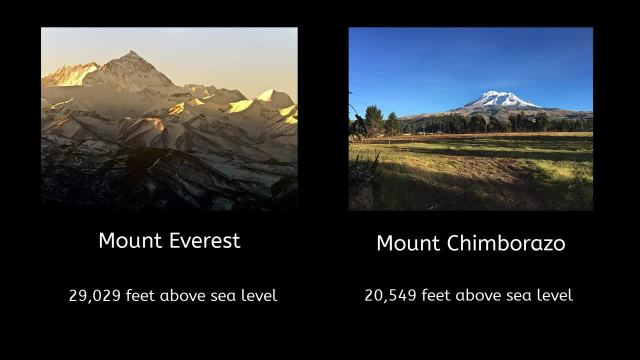 is located just one degree 28 minutes south of the equator, Earth's fattest point. it gets a boost of some 13 miles further from the center of the Earth, which puts its height at 3,967 miles from the center of the Earth, two miles more than the distance from the. 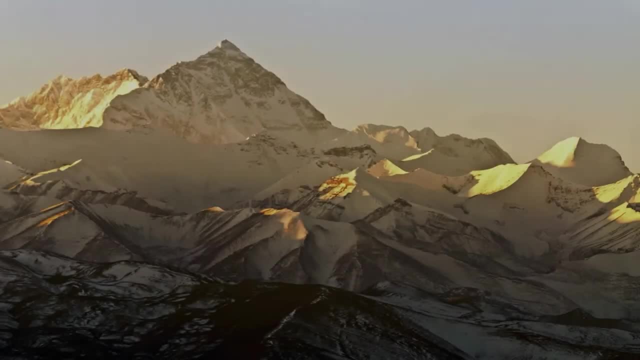 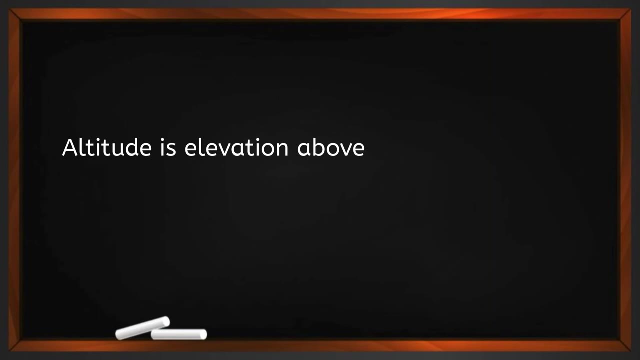 center of the Earth to the summit of Mount Everest. Don't worry, Mount Everest fans. Everest is still the highest point on Earth in terms of altitude, meaning its summit's elevation above sea level. Geologists will tell you that the Earth has essentially three. 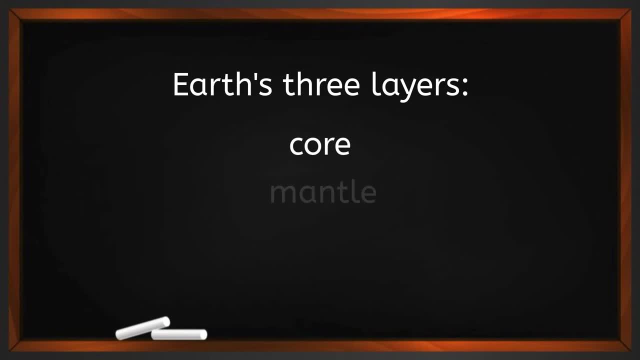 layers: The core, made of hot iron and nickel, the mantle, a thick layer of rock. and the crust, Earth's thin rocky surface, And we'll get into that later, But for this lesson it's important to understand that the different elements of the Earth's natural environment 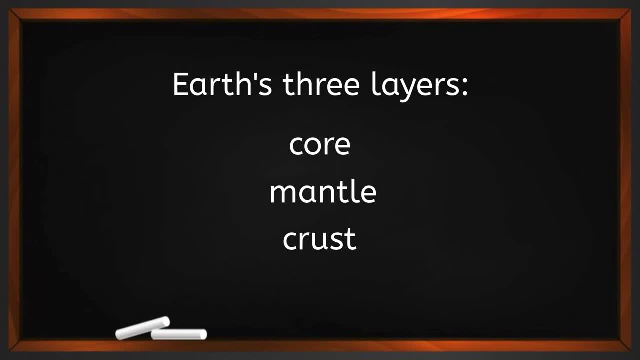 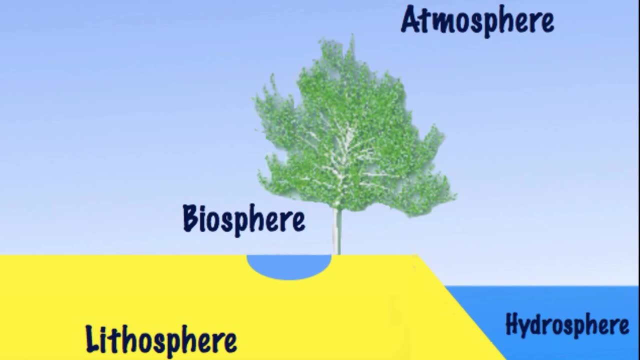 are often thought of as a set of related spheres dominated by particular physical forms. What does that mean? Soil, rocks, landforms and other features on the Earth's surface make up the lithosphere. The layer of air, water and other substances above the surface make up the atmosphere. 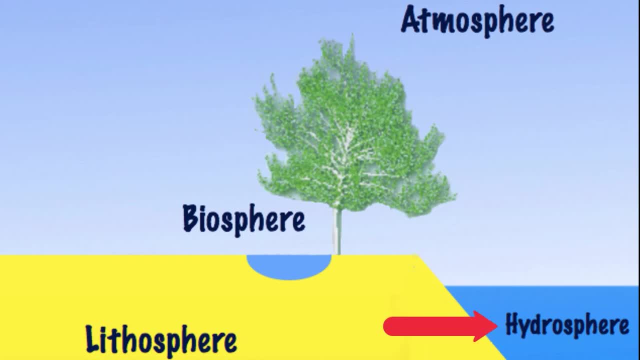 Water on the surface, underground and in the air make up the hydrosphere. The biosphere is made up of the parts of Earth where life exists: the world of plants, animals and other living things that live in the land and water.